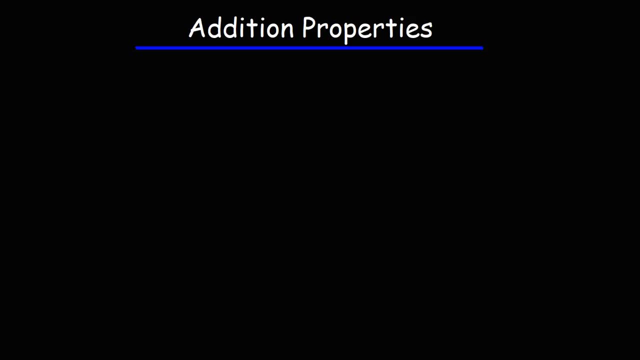 In this video we're going to talk about a few addition properties, particularly the commutative property of addition, the associative property, the inverse and the identity property of addition. So let's go ahead and begin. Let's start with the commutative property. 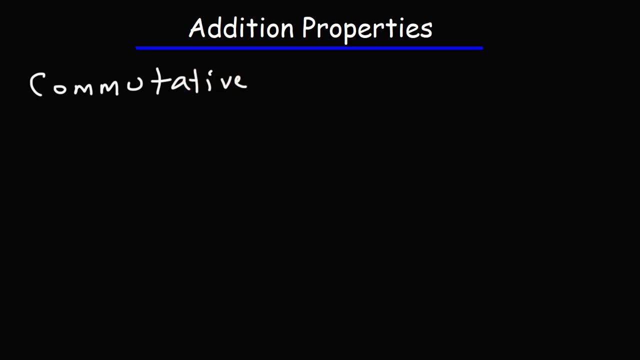 of addition. Here's the formula that goes, with that A plus B is equal to B plus A. So what does that mean? The order upon which you add two numbers doesn't matter. The value will not change. It will remain the same. So let's say A is 5 and B is 3.. 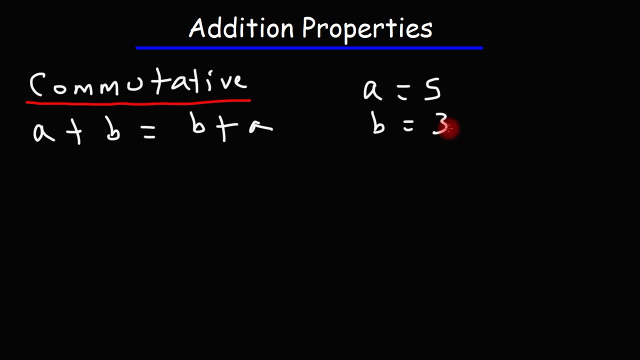 5 plus 3 and 3 plus 5 will give us the same value. 5 plus 3 is equal to 3 plus 5.. So if we add 5 to 3, we get 8.. If we add 3 to 5, we also get 8.. The value remains the same. 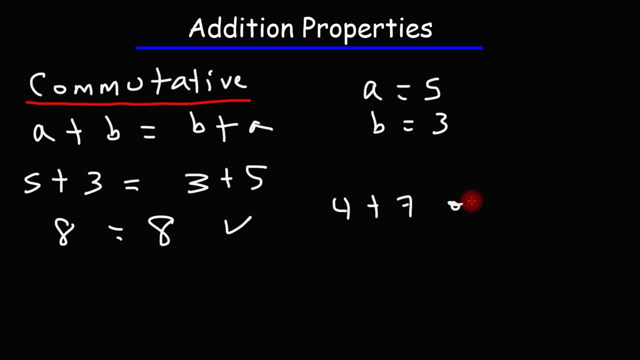 So, for instance, if we add 4 plus 7 or 7 plus 4, we're going to get the same answer: 4 plus 7 is 11 and 7 plus 4 is 8.. So we're going to get the same answer. 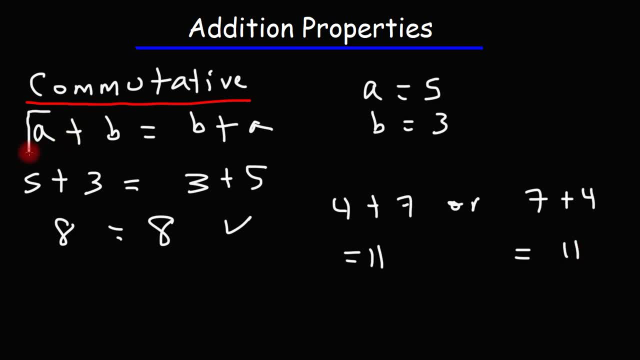 So, for instance, if we add 4 plus 7 or 7 plus 4, we're going to get the same answer: 4 plus 7 is also 11.. So that's the basic idea behind the commutative property of addition. 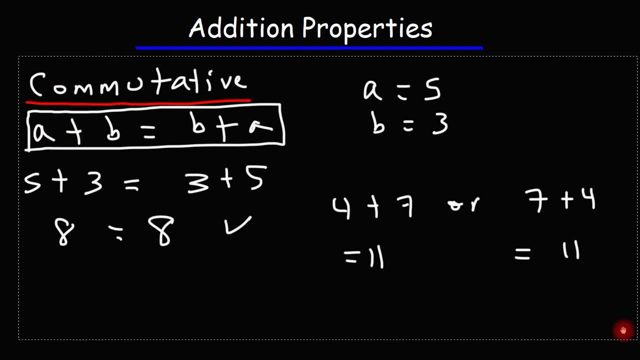 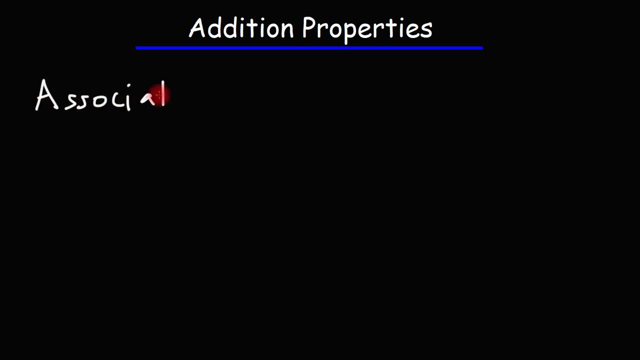 A plus B is equal to B plus A. Now let's move on to the associative property of addition. The formula that goes with that is this: A plus B plus C is equal to B plus A. A plus B plus C is equal to A plus B plus C. 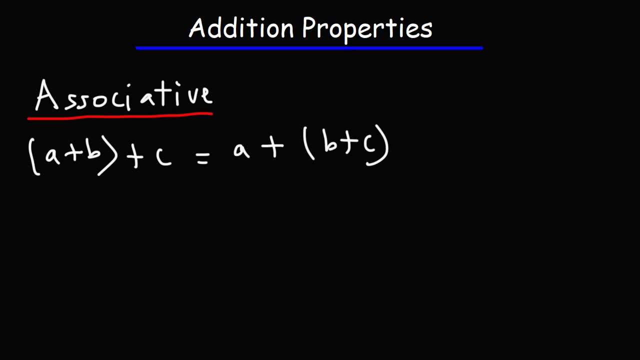 Now, when you're only adding numbers, the order upon which you add doesn't matter If you're just only adding numbers, and that's a big if. Now, when you're working on math and you're following the rules of the order of operations, 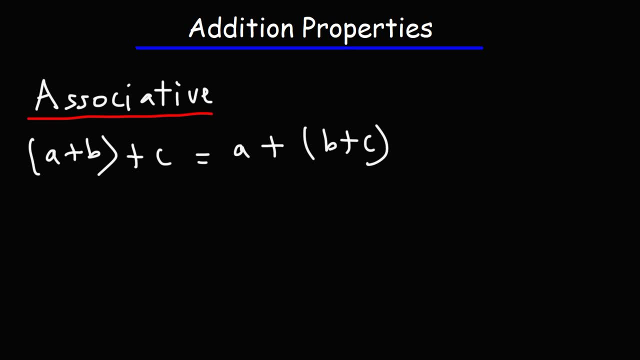 PEMDAS, typically you would work inside the parentheses, So we're going to do an example of that shortly. Let's say A is 3.. Actually, let's use our old values. We're going to say A is 5,, B is 3.. C, we're going to make it 4.. 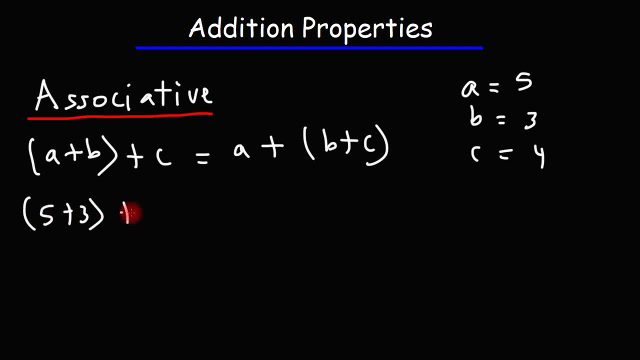 So we have A plus B, that's 5 plus 3.. And then we have a C value And then A, and then plus B plus C. So let's work inside the parentheses first, 5 plus 3 is 8.. 3 plus 4 is 7.. 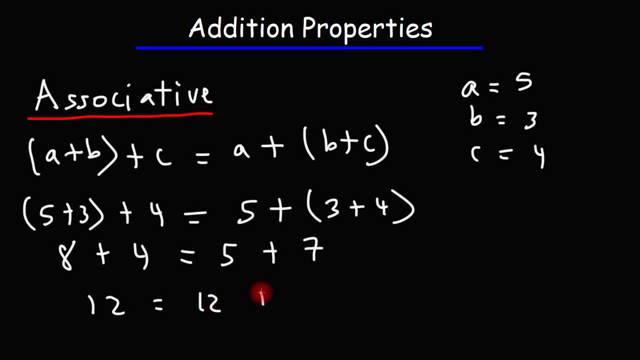 8 plus 4 is 12.. 5 plus 7 is also 12.. So, once again, it doesn't matter the order of which you add things. If you're only adding, the value will remain the same. Now let's move on to the identity property of addition. 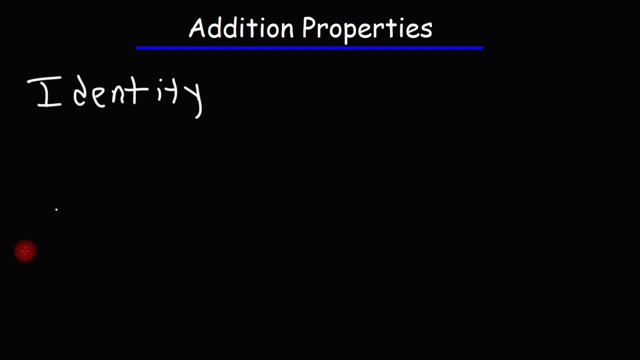 The formula associated with this is: A plus 0 is equal to A, Which means if you add 0 to anything, you're going to get the thing that you started with. Adding 0 to a number doesn't change the value of that number. 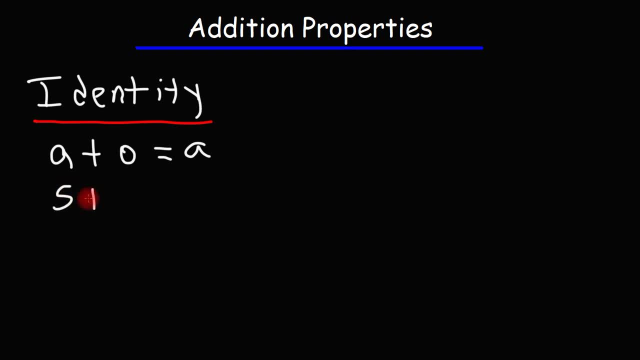 The value remains the same. So if we add 0 to 5, we're going to get 5.. If we add 0 to 5, we're going to get 5.. If we add 0 to 5, we're going to get 5.. 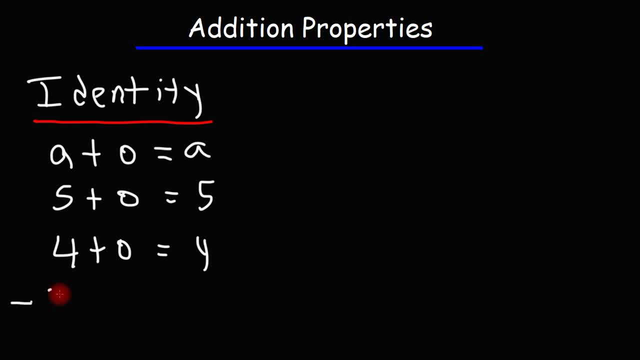 If we add 0 to 4, we're going to get 4.. If we add 0 to a negative number, like negative 3, we're still going to get negative 3.. So that's the identity property of addition. 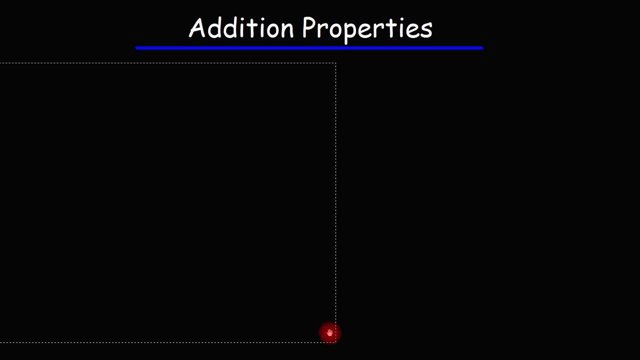 A plus 0 is equal to A. Now let's talk about the inverse property of addition: A plus negative A. A plus negative A is equal to 0. In other words, negative A negates the value of A. They cancel each other out and they become nothing.